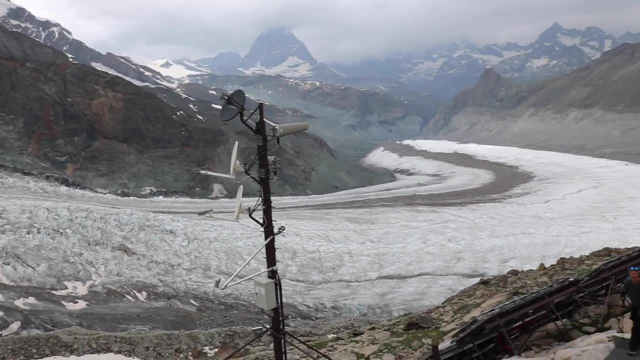 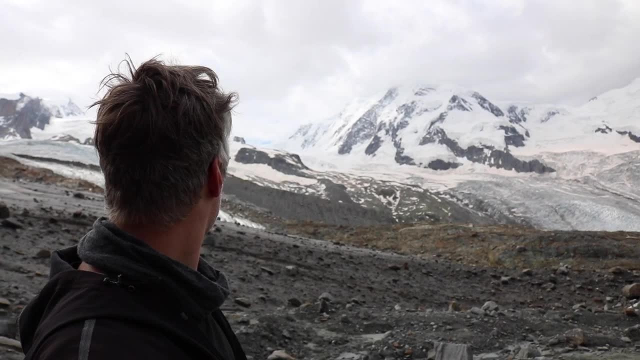 We are at Switzerland's second largest glacier, a system called Gorna Gletscher. It's a glacier that produces ice very high right there, next to the peak that we see over there, which is the highest peak in Switzerland, called the Dufour Spitze. 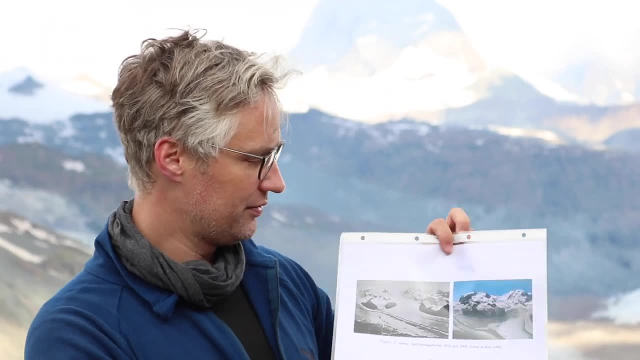 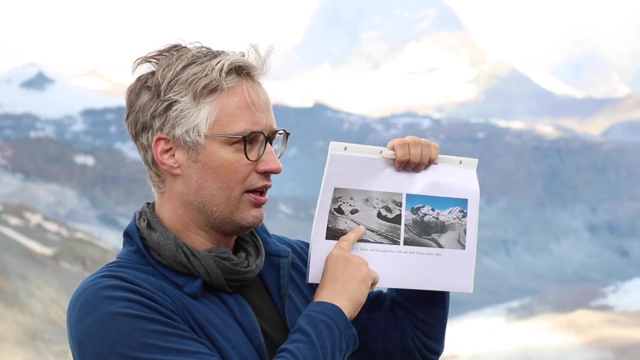 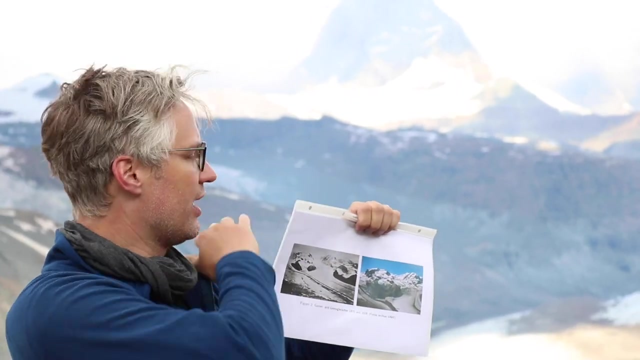 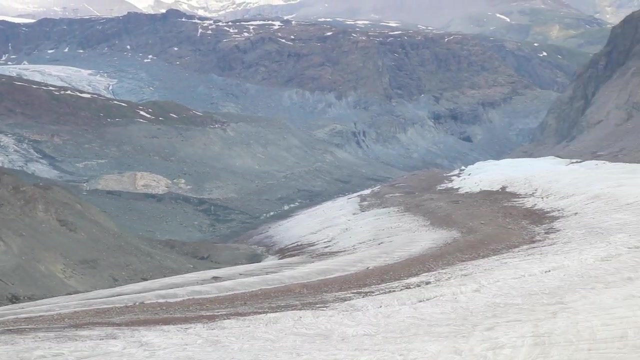 This picture is quite nice because it shows you a before-after image. This is from the 1870s, so about when the little ice age was ending. So really, the last extent from where we see all these lateral moraines. This is in 2006,, and you see right now how it is in 2019.. 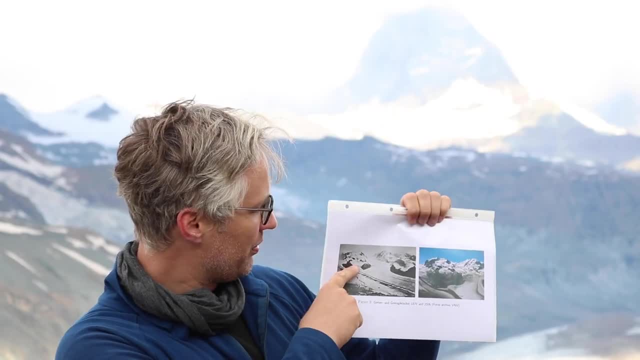 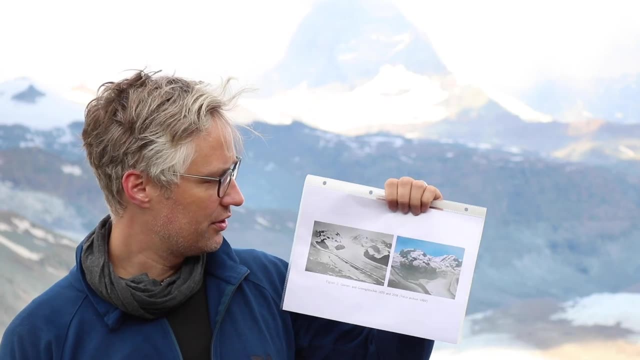 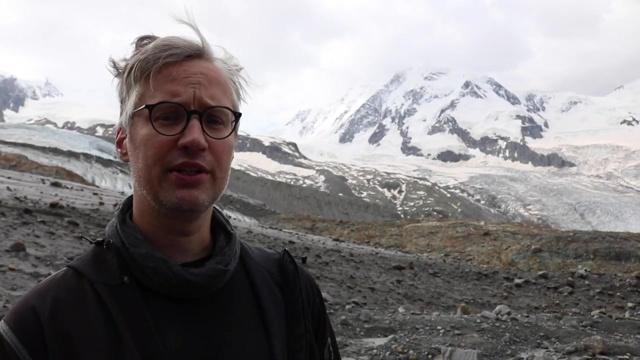 So you can see that 150 years ago, where we were, there was ice flowing down right here from the central glacier, the Monte Rosa glacier, and it was still attached to the glacier down there. What we studied here in particular was the drainage of an ice-marginal lake. 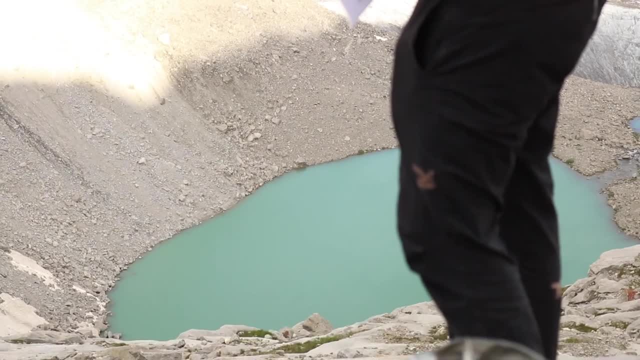 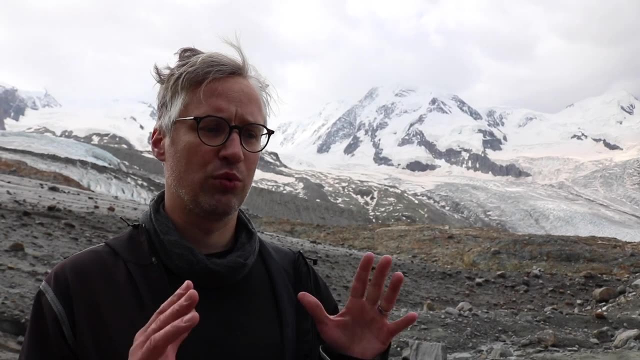 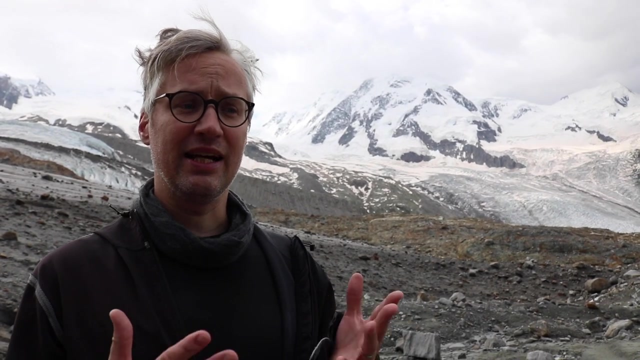 This is a typical phenomenon which you basically have everywhere in the world where you have glaciers that melt. The problem is that you have a water body which is at least partially damped by an ice body, and these ice dams are inherently unstable. Ice is not a very reliable damming material. 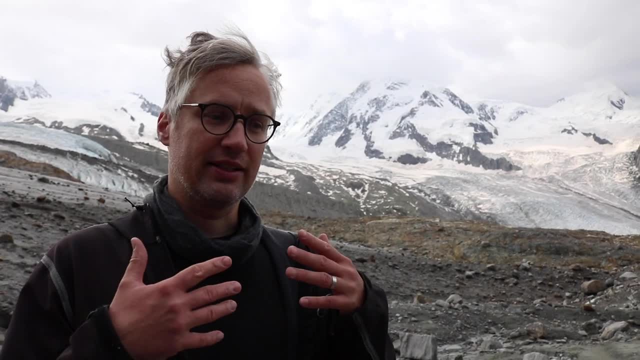 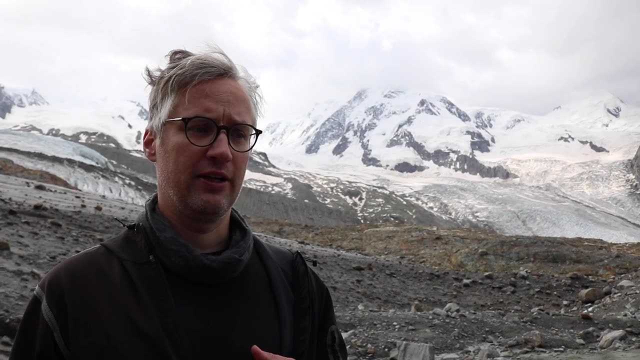 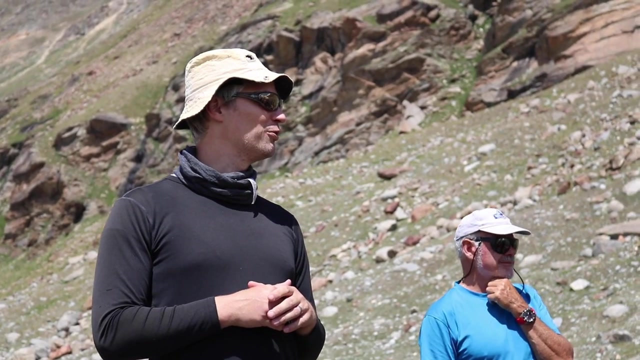 And so regularly these lakes outburst, they find a way through the ice or they can break the ice dam and they produce floods in downstream communities. So the name is Jokull Hallopp. What Jokull Hallopp? which is the Icelandic? it's an Icelandic term. 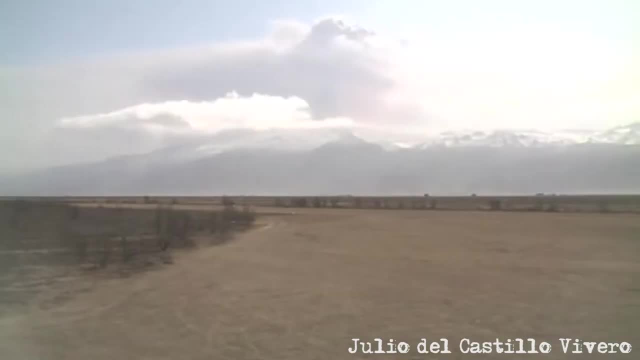 Jokull, you may have heard this, that's glacier like Eyjafjallajökull, the volcano, Yeah And Hallopp, and you actually it's a. you have an L, an H and an L. 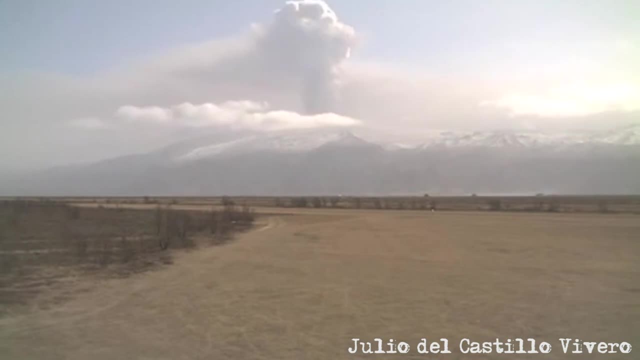 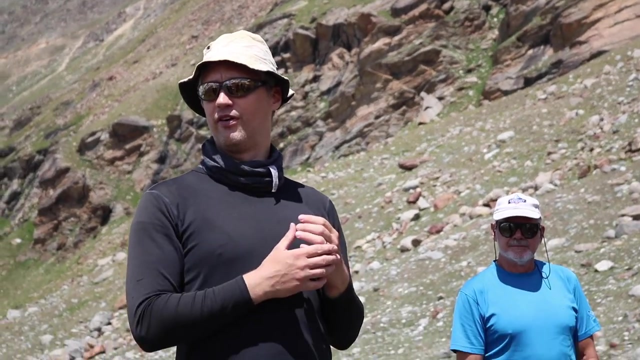 And an Icelandic person once told me you pronounce every single letter, so you really do say Jokull Hallopp, And the Hallopp means sprint, So it means glacier sprint And you can see the evolution of these lake basins right here. 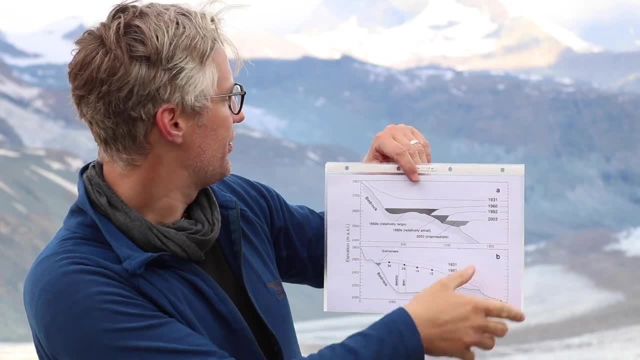 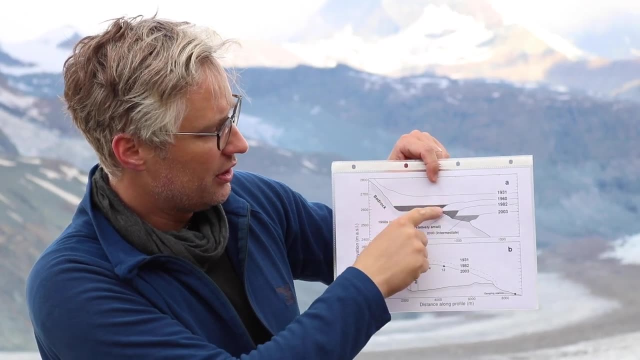 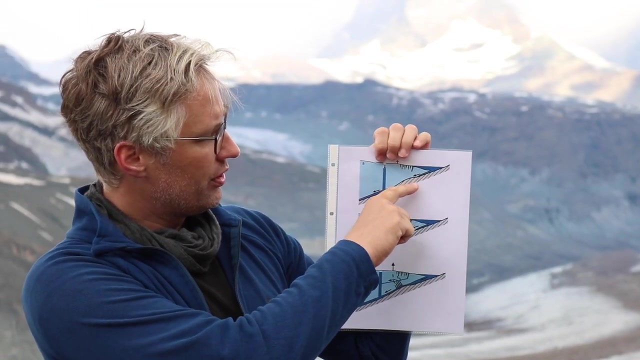 So we're standing somewhere right here. This is the glacier over there And you can see how, as the glacier surface was lowering, you were starting to get this depression right here, which was then filled with the lake water, And these lakes start draining when the lake water is capable of. 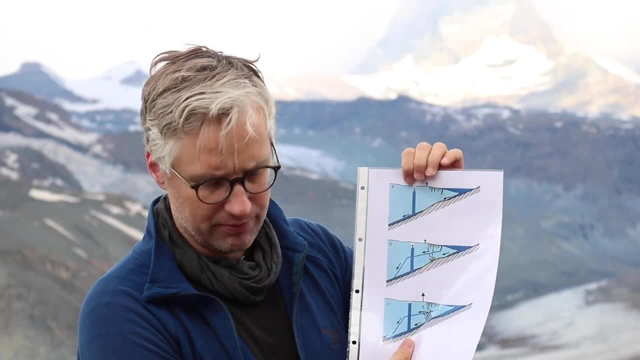 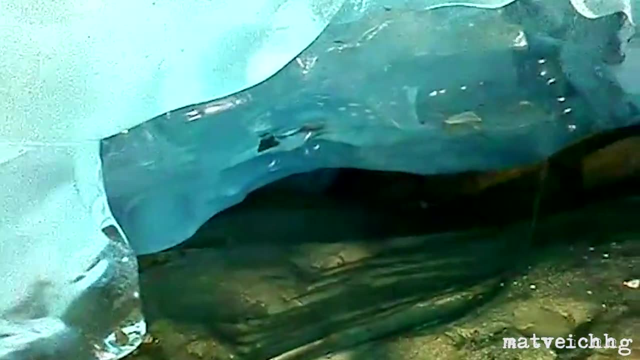 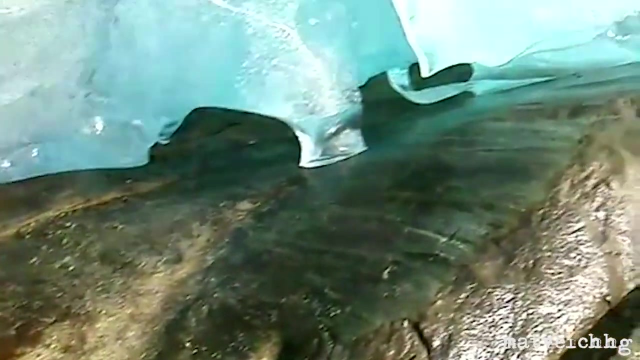 accessing the subglacier drainage system. So you can imagine, below these ice tongues in the summer you have very large channels. They can be two meters in diameter And these channels are very efficient, So as soon as water or lake water is pressed through them, 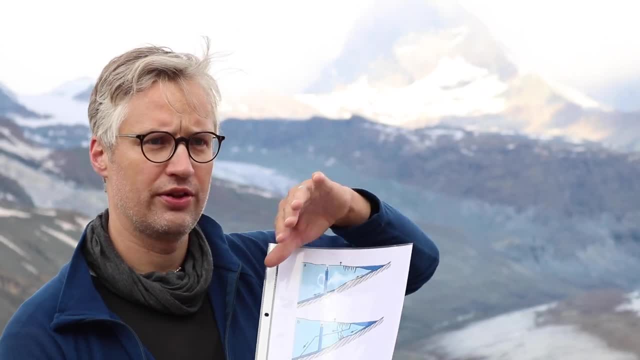 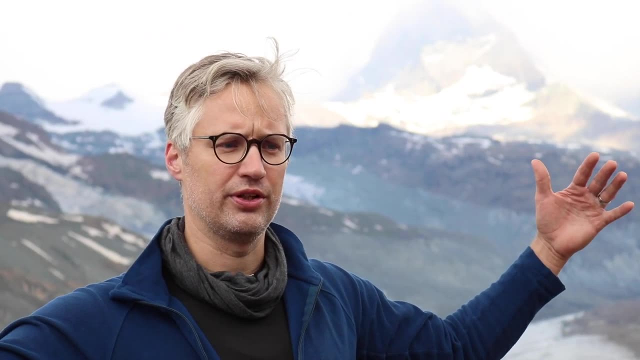 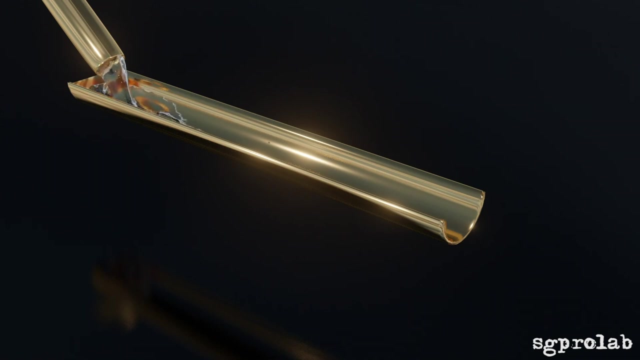 they also water. They also widen because as water flows along the ice walls there's friction that's dissipated And this friction increases the diameters very rapidly. Flow of water through ice wall channels is actually a very interesting problem. The hydraulic engineers they're familiar with water flow through pipes. 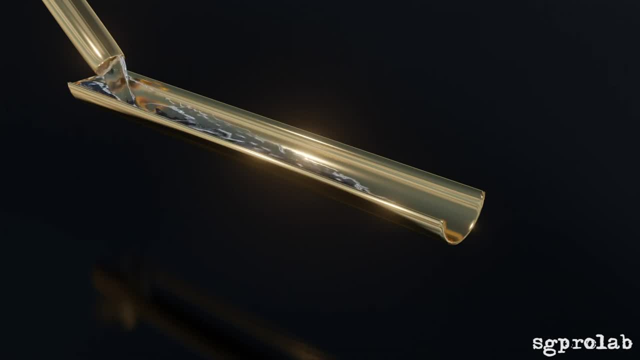 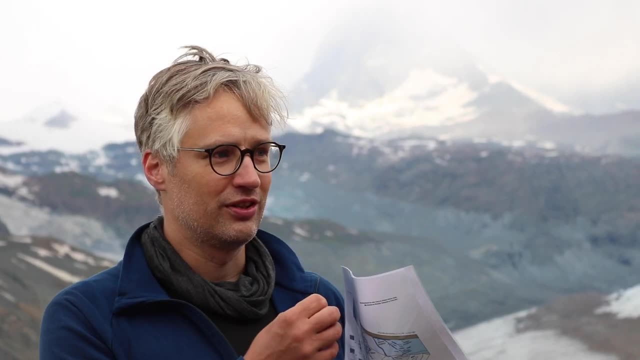 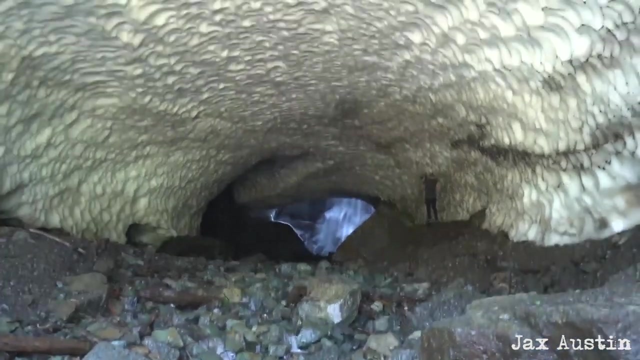 but they usually calculate water flow through metal pipes or concrete pipes which don't erode For glaciers. you have the interesting case where the water is the same material as the channel walls, It's just the solid state. But of course what can happen is the water can melt the pipe. 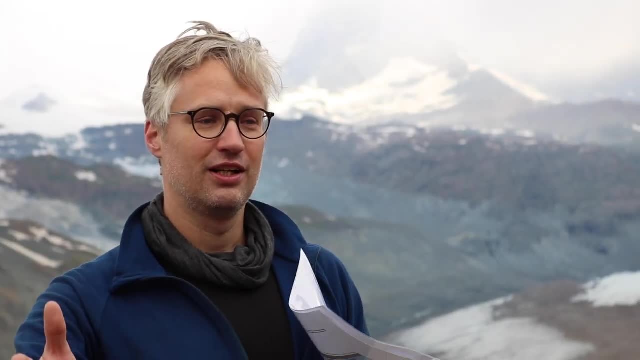 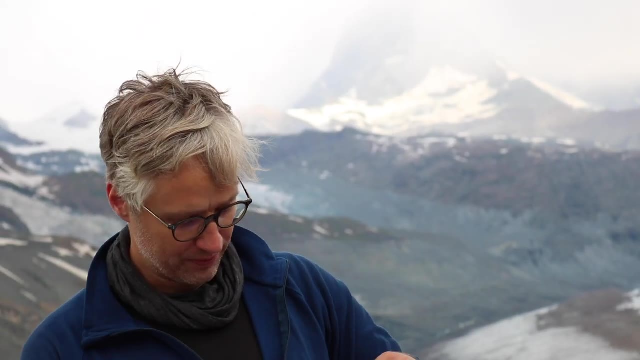 make it bigger, and this melt water contributes then to the flux. It can also freeze to the walls, which makes the walls shrink. So it's actually a quite mathematical problem. But the glacier doesn't always do the textbook example. Of course you can also have, a lot of times, crevasses. 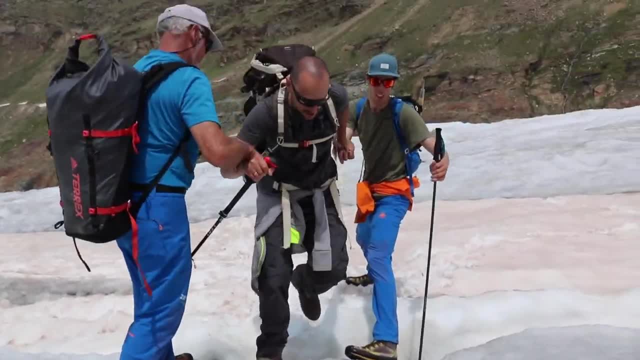 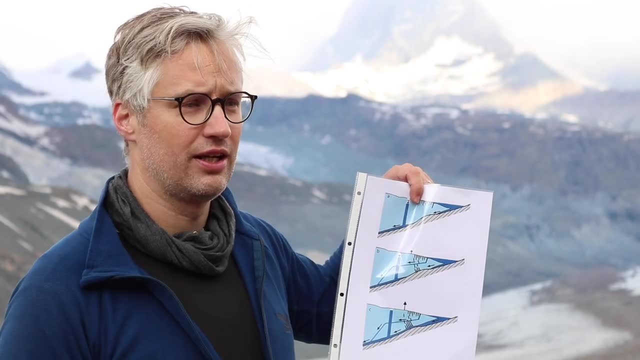 which somehow route the water and glacial To a moulin, which you see right here, and then to the subglacial drainage system. And what you can also have, and this is what everybody is afraid of- is if you have lots of crevasses right here. 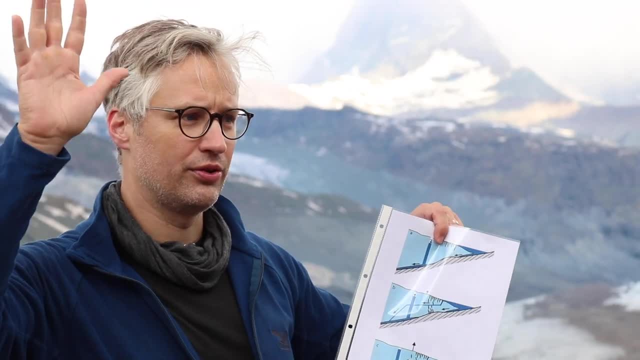 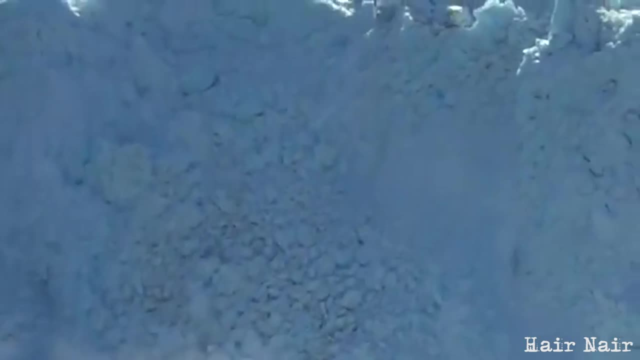 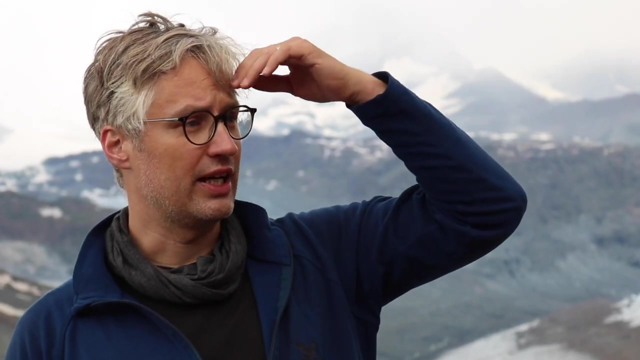 and this entire part starts floating up. so you have an iceberg calving event and this is a matter of seconds or a minute, and then all of a sudden, you have a huge connection And these are the most dangerous drainages That happened in the valley next door in the 1960s. 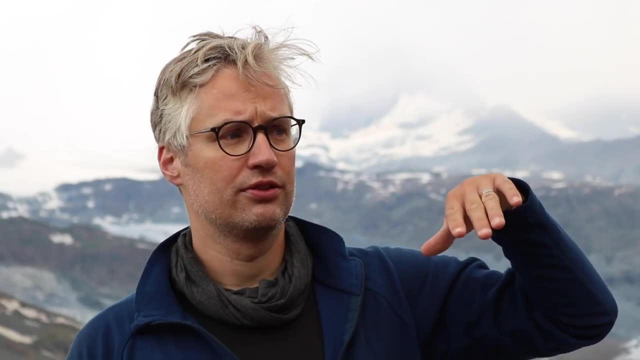 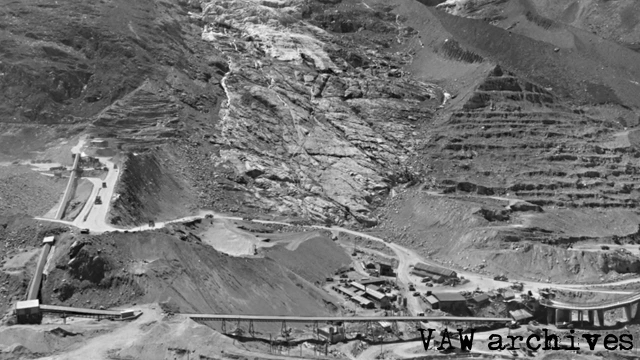 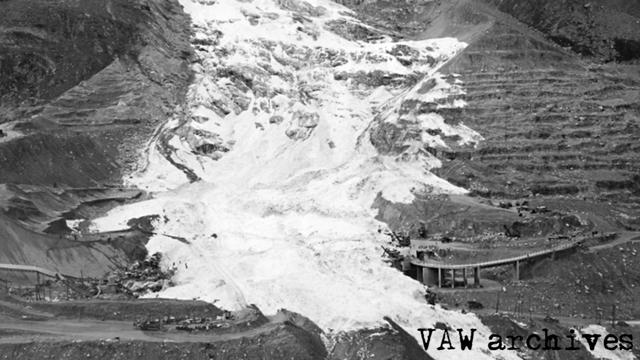 There was a glacier in a steep topography step, just like this one right here, and there was a construction site underneath the glacier, And then, all of a sudden, the tongue collapsed. It killed 88 construction workers, which were completely surprised. A lot of research was initiated, of course, to understand this event. 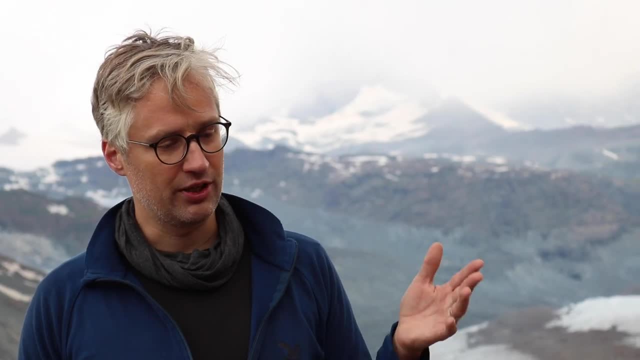 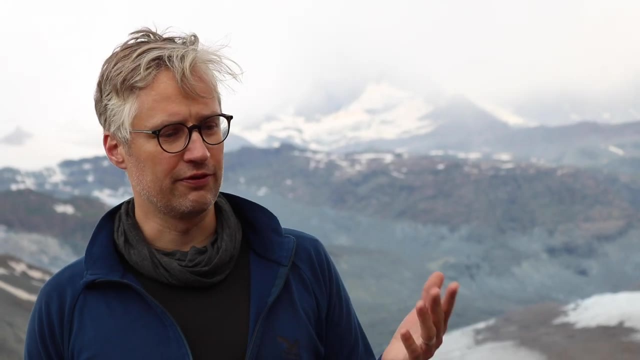 and it was noticed that it's not uncommon even for steep glaciers to speed up when there's a lot of melt. but if the drainage system is unfavorable, when it cannot evacuate enough melt, then too much pressure builds up and the whole thing goes. 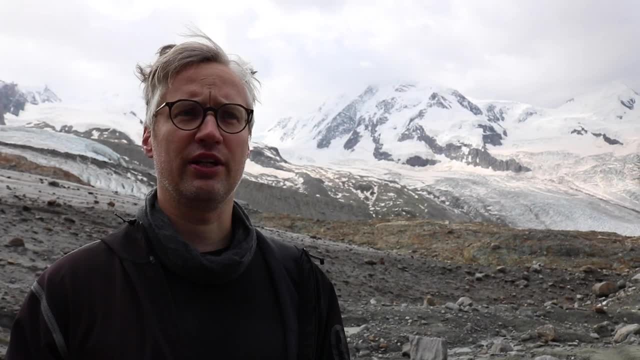 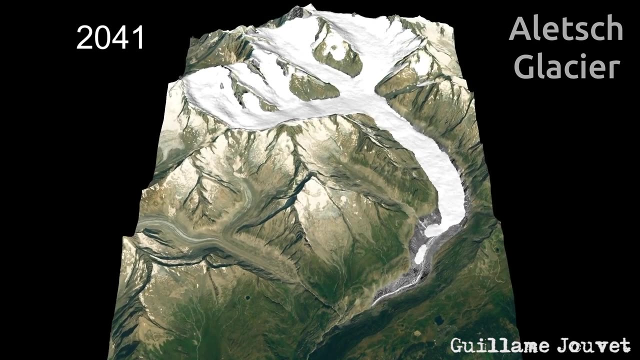 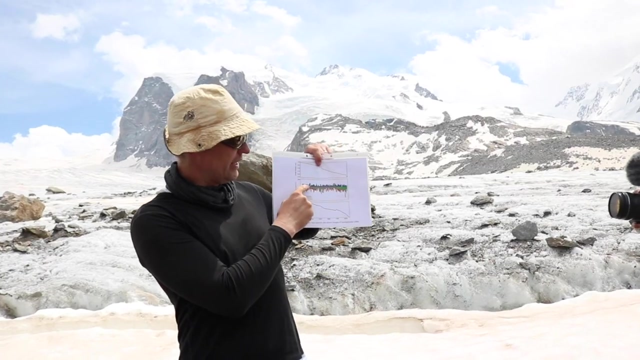 In general. you see, the glaciers are receding. in Switzerland, The parts of the glacier that gain mass are smaller and smaller and the parts of the glacier that melt over average, over a year, are bigger and bigger. This plot, which is the mass balance in the winter. so how much mass is gained? 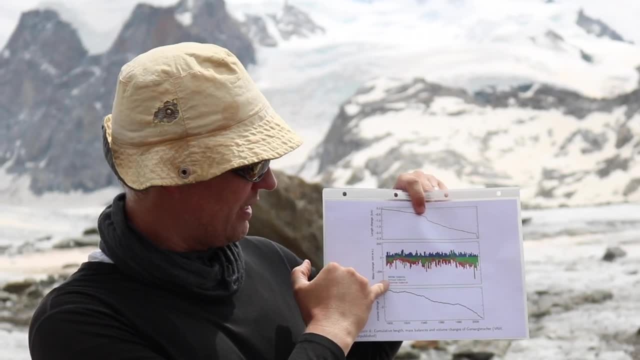 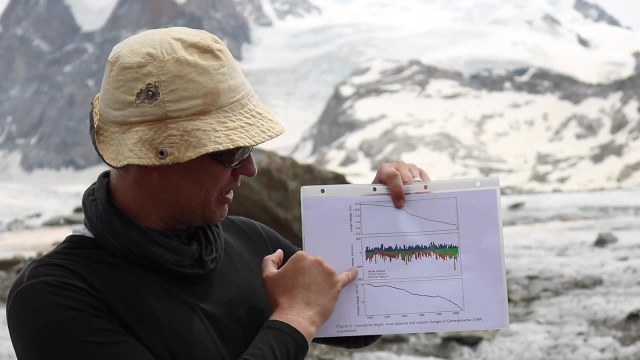 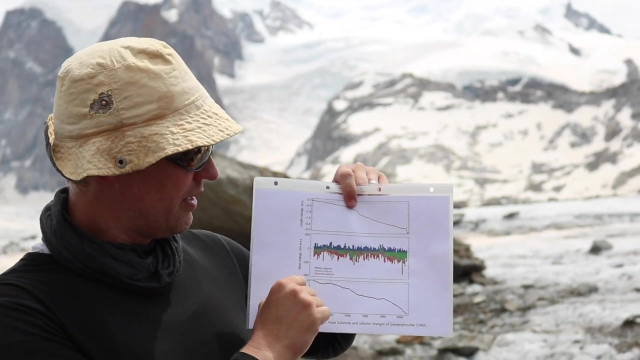 the mass balance in the summer, which is red, and the whole balance, so one minus the other. You can also see that it's been the annual mass balance here. the green bars, they're consistently negative for almost all years. But what you can also see, it's really the summer balance. 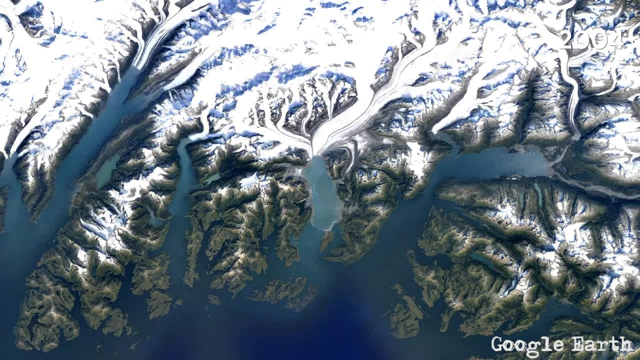 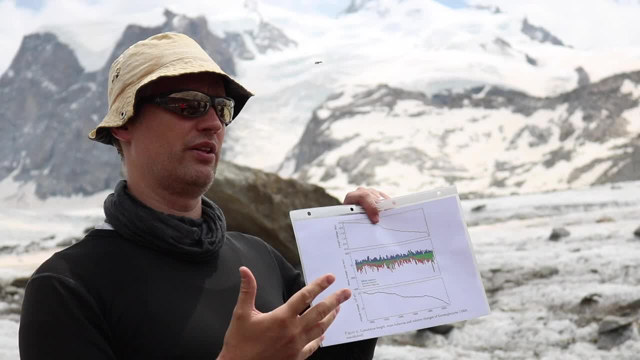 the negative summer balance that's picking up right here. It's not that the glaciers don't get as much mass in the winter anymore. Here in the Alps it's really the summers really hit the glaciers. This is really what's kind of the daily bread of glaciology. 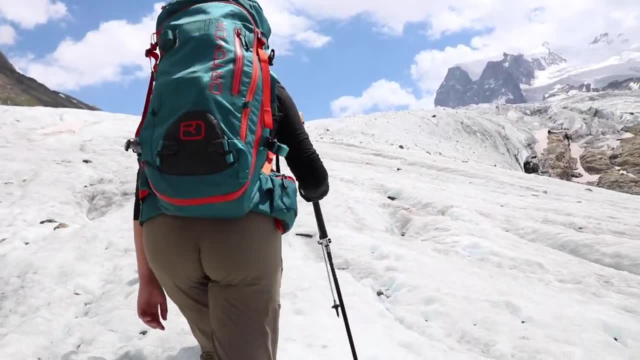 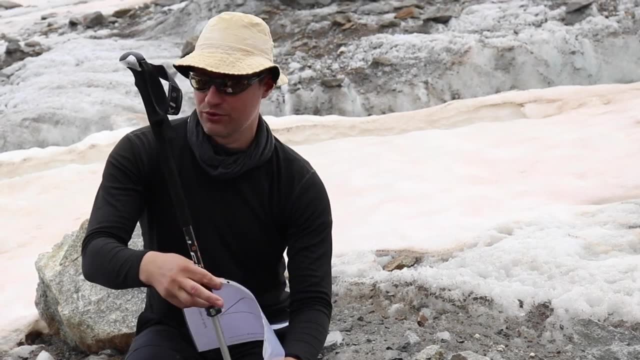 You take a pole and you drill it into the ice, maybe 10 centimeters or a bit more, And then you can come back regularly and see where the ice surface is. So when you drilled it in, for example, the ice surface was here. 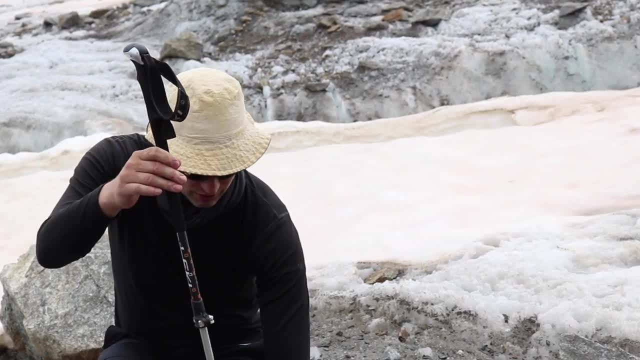 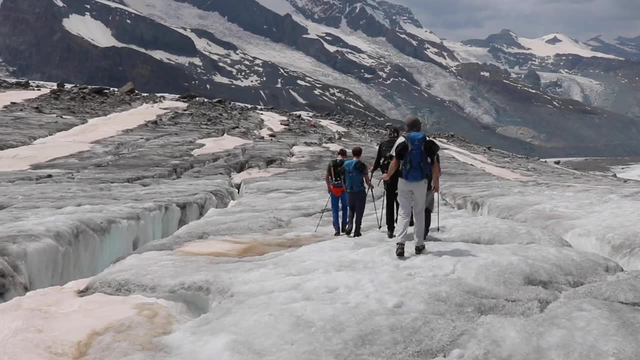 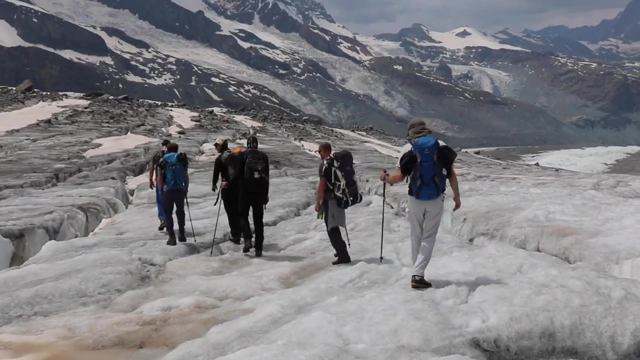 Then you come back two weeks later. the ice surface is here, and so on. Then you come back in the winter. the snow surface is up here And this is what glaciologists use to to measure the specific mass balance. So the mass balance that's very specific to a certain location. 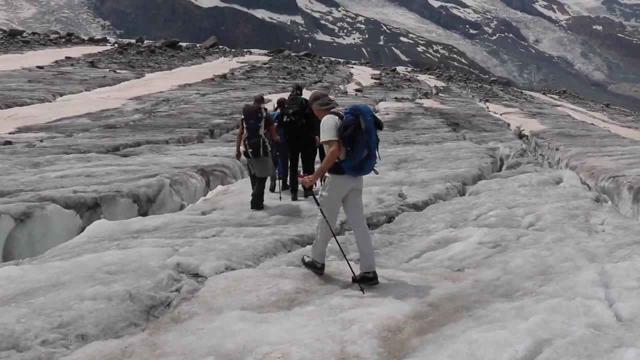 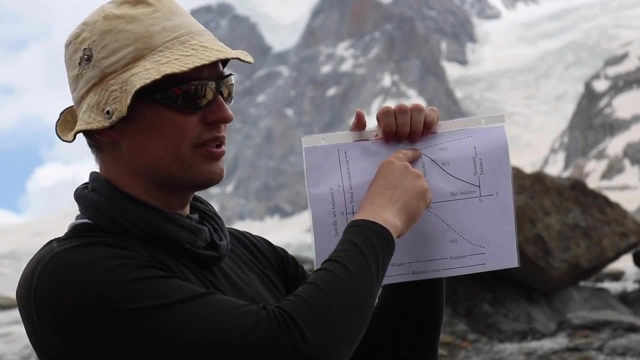 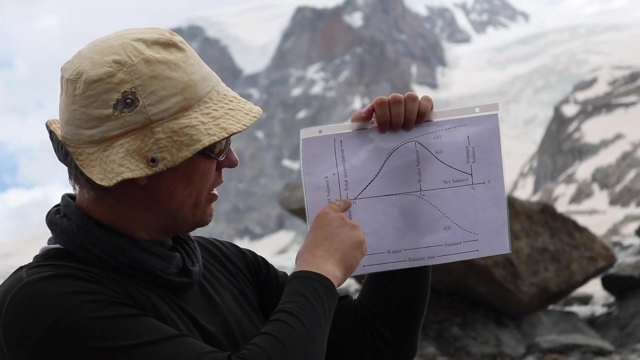 And then you produce these plots, You have the accumulation in the dotted line right here, which in the winter increases rapidly. You get lots and lots of snow, And then in the summer you stop or you get very, very little snow. At the same time, you get almost no melt in the winter. 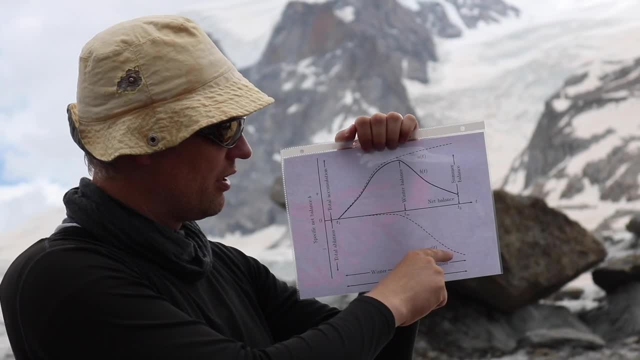 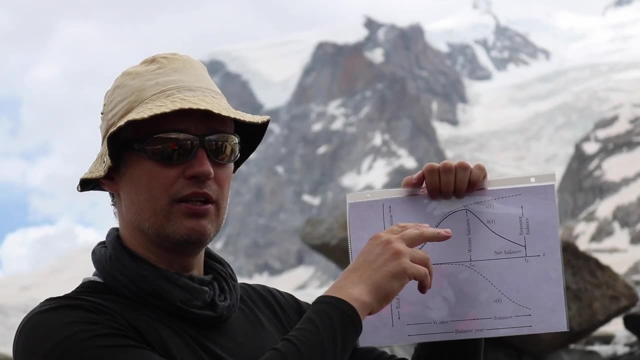 And then, towards the spring, the melt picks up Right here, And then, once we get into fall, the melt slows down again And the balance, the entire balance, is simply the algebraic sum of the two, which is the solid line right here. 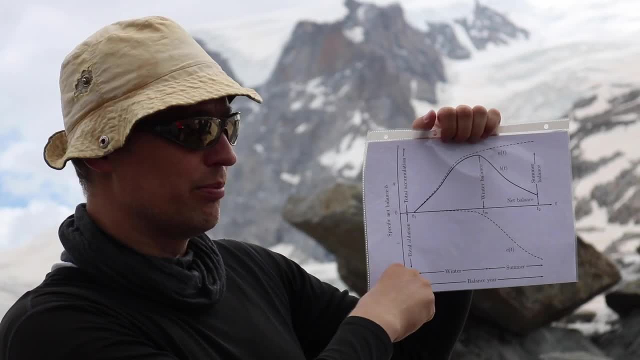 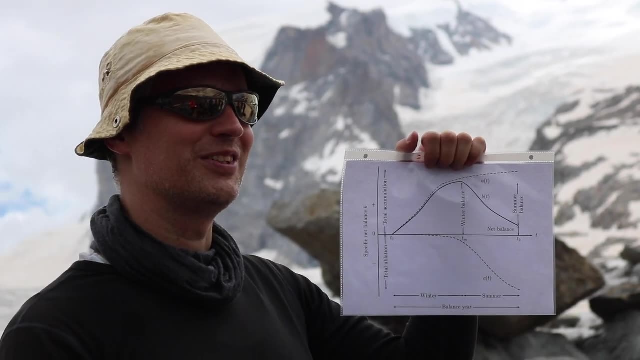 So if you look at the solid line, this right here is the total ablation, the mass loss. This is the total accumulation, the mass gain. Then you know where you are on the glacier. Does anyone, can anyone, say, Are you in the ablation zone or the accumulation zone? 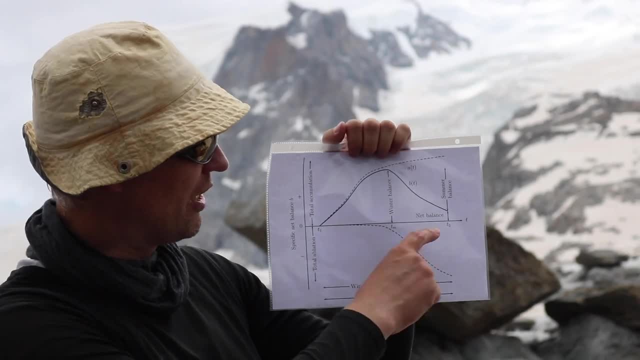 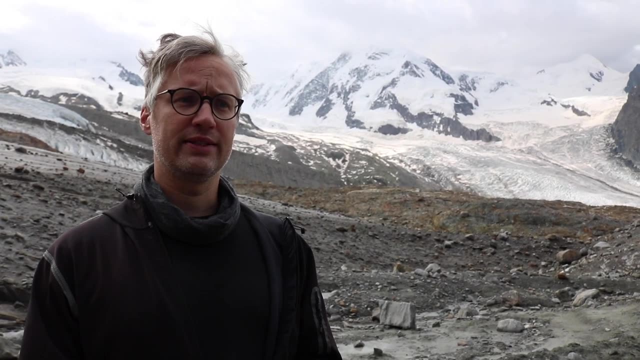 Ablation, No, sir. Ablation, No sir, That's accumulation. Yes, Because you have a positive mass balance at the end of the year, so you're in the accumulation zone. There are several concerns. One is that the glaciers are really helping us these days. 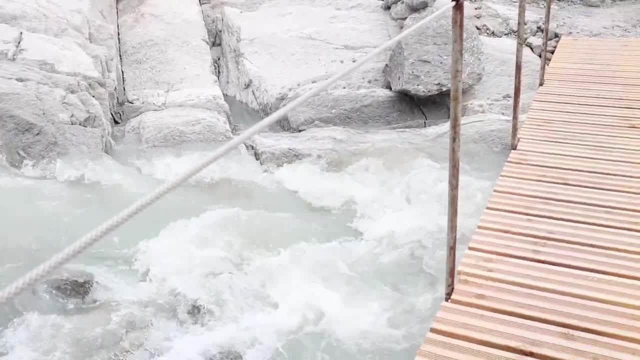 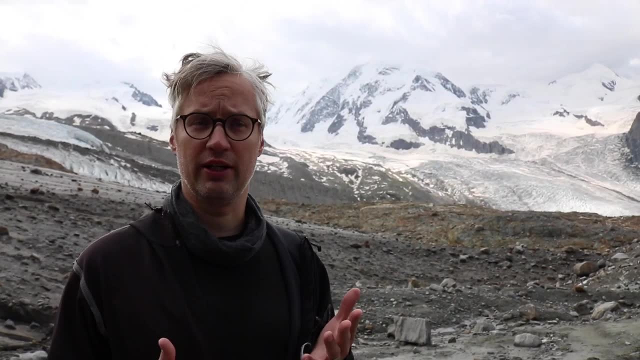 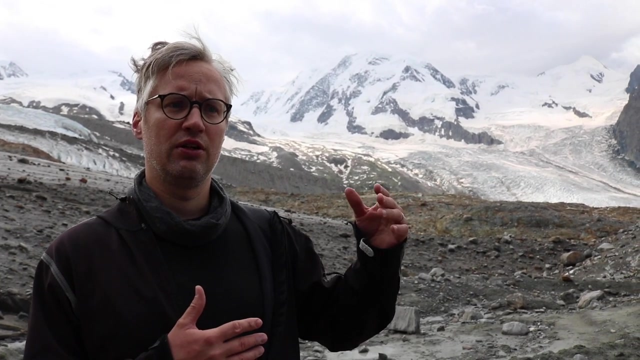 because when we have a very dry and hot period in the summer, without lots of rain, that means that the rivers carry less water And the glaciers, in this moment they melt, So they kind of make up for the lack of The lack of water due to rain, and so this is a damping factor. 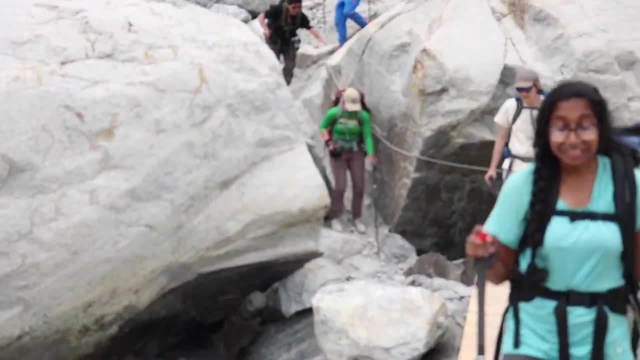 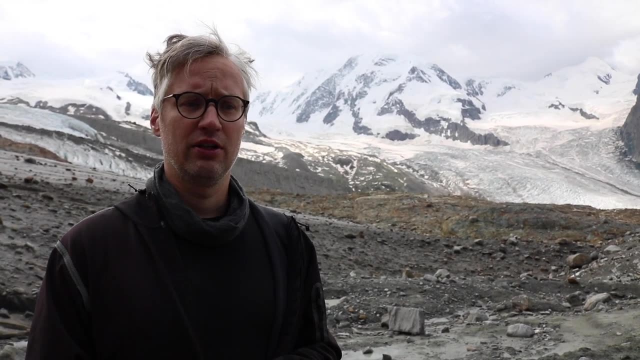 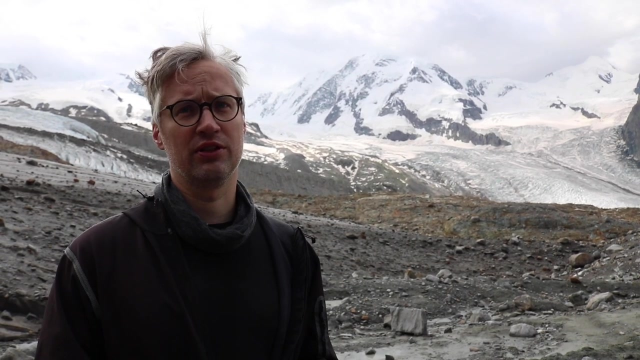 In the future. when we have less glaciers or when glacial basins start to be ice-free, we don't have this damping effect And this means that when we have precipitation, we have lots of water. When we have no precipitation, when there's a drought, we have little water. 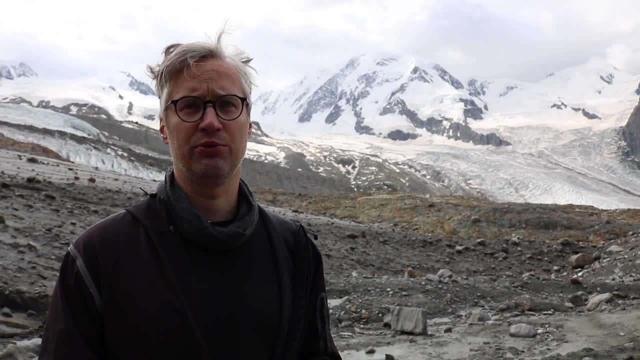 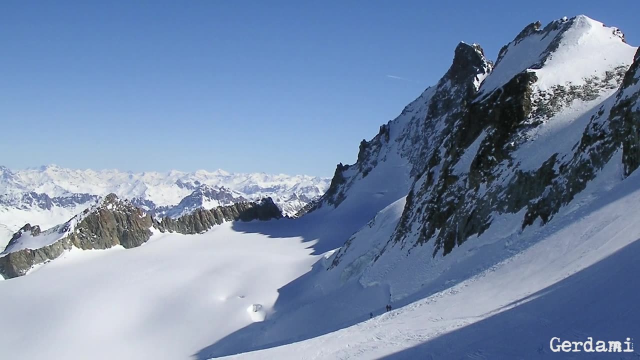 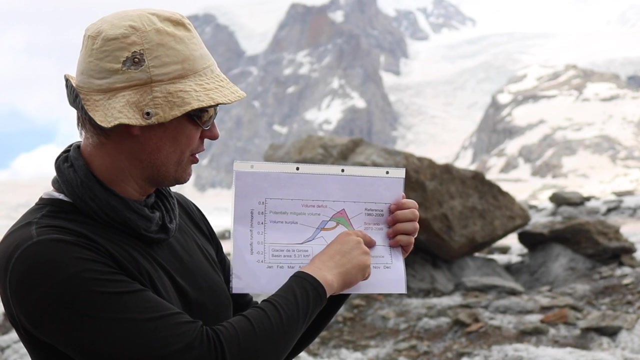 And this is something that's certainly of concern for water. This shows you how this runoff will change. This is a small glacier in France. The solid line, the solid black line right here, shows you how the runoff from this glacier, so the entire melt on the glacier, was in a reference period 1980 till 2009.. 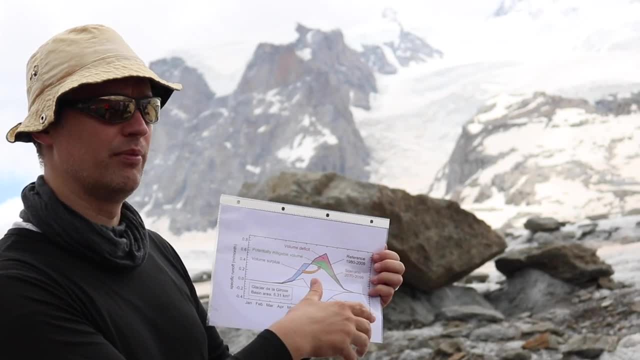 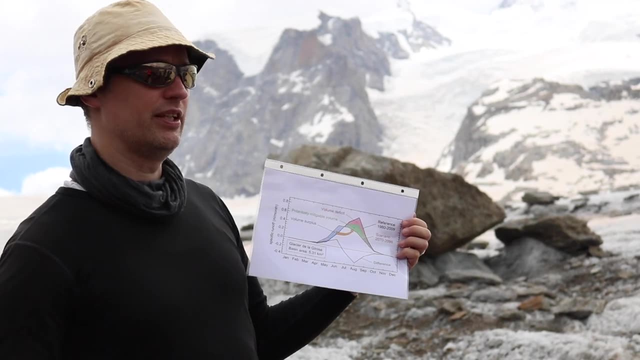 You see what you expect in August, when it's the hottest, All the snow, the protective snow, is gone. That's when you really get the high melt rates. And now what happened? If things keep going like this, if the glaciers get smaller, of course, this will change. 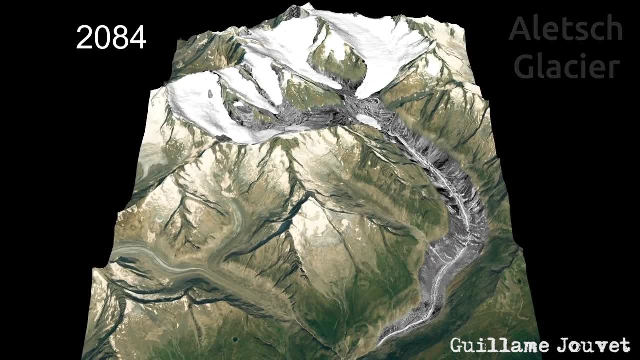 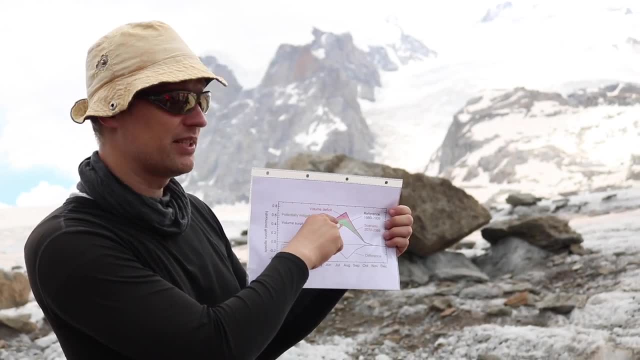 And the red line right here shows you the projections for the year 2070 to 2099.. And you see that, first of all, we have less runoff. The runoff peaks are lower. They're projected to be lower by around 10 percent annually in the summer. 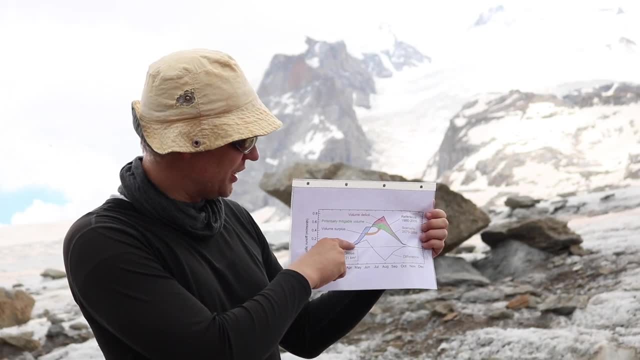 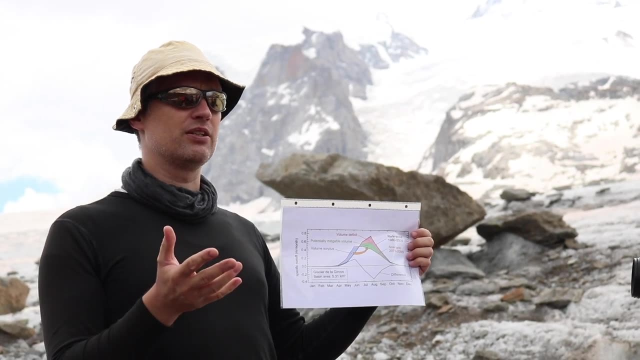 perhaps even by almost a third. But what you can also see is the runoff peak occurs earlier in the year And this is easy to understand because the glaciers- when we have a dry, hot summer, the glaciers are very useful: They melt. 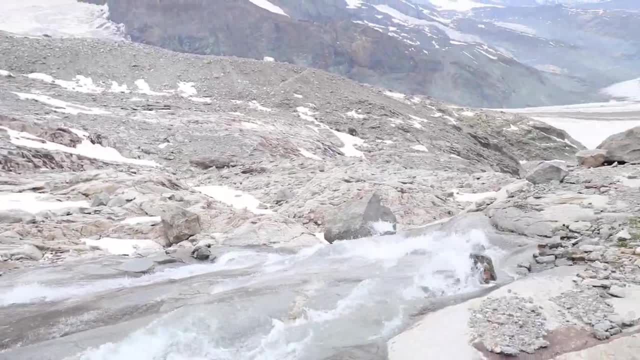 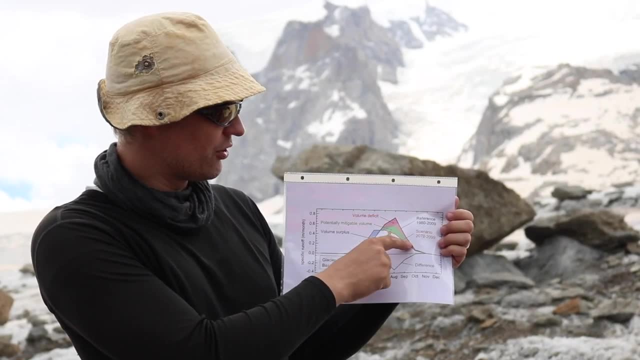 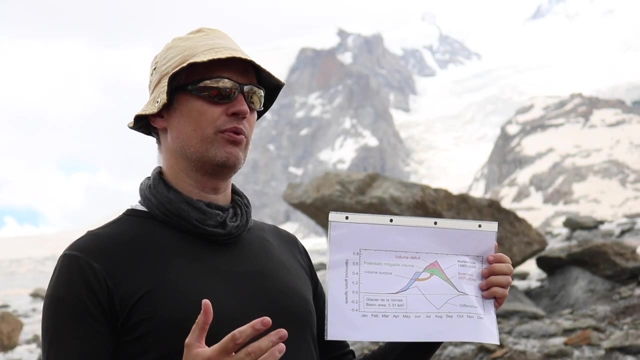 They give us water in the rivers when there's absolutely no precipitation. When the glaciers are gone, then we don't have this effect anymore. This entire area is then how much we will lack how much water. But this area right here also tells you how much water we will get at a point when 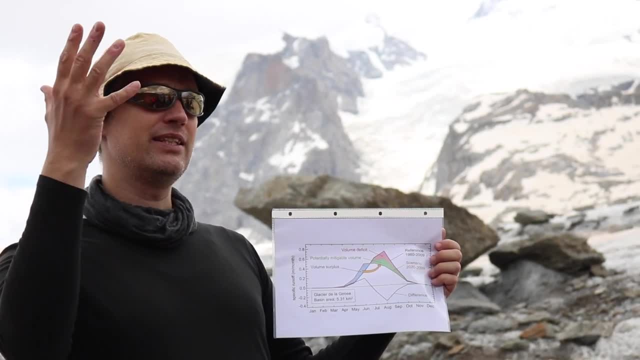 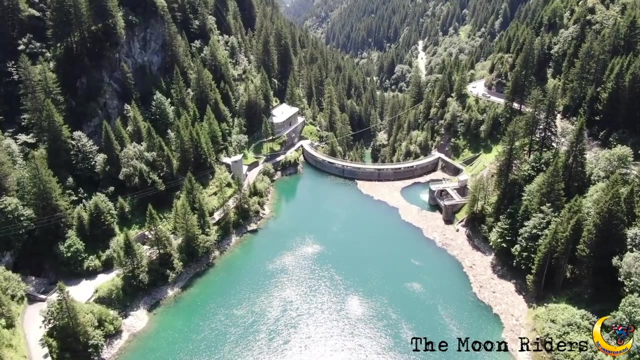 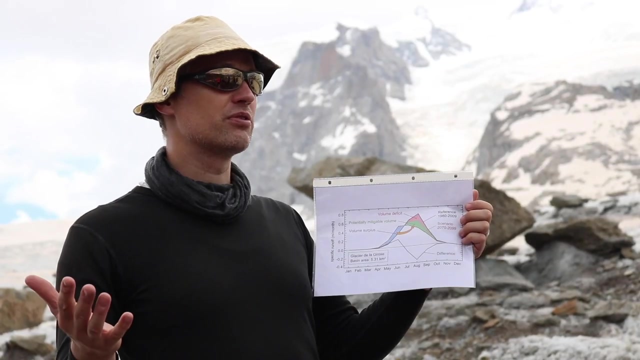 before we didn't have as much water. So the question is: can we somehow take this water, which we've been able to do without in the history, and just make it release to the valleys a little bit later? And the way you would do this is by constructing dams, of course. 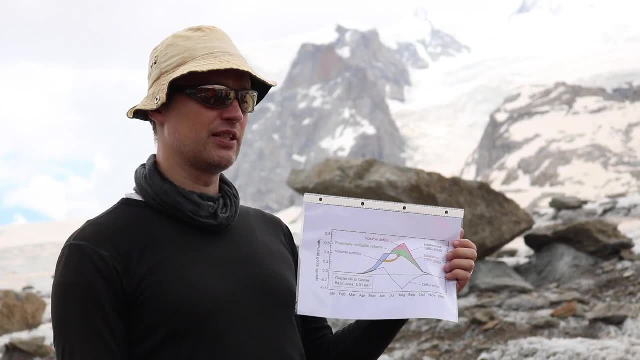 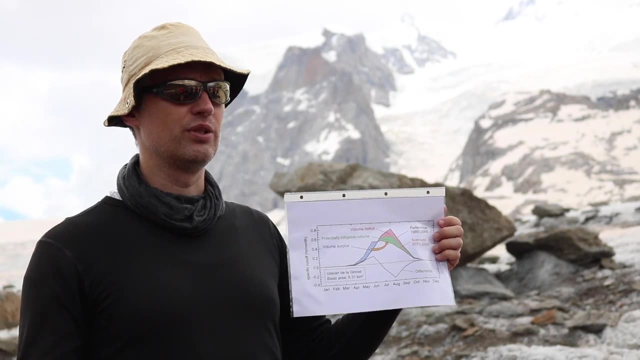 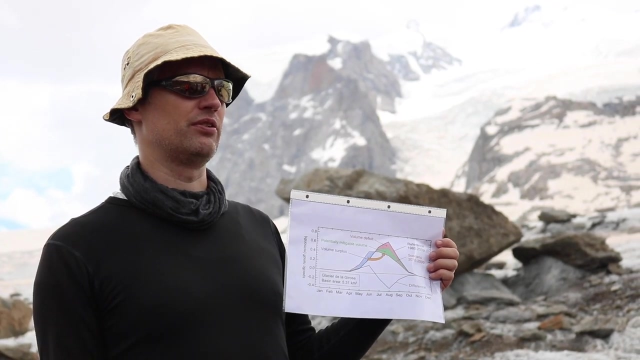 And it turns out that you cannot mitigate this entire difference, but perhaps around two-thirds of it, And this would require the constructions of half a dozen to a dozen dams, and that would be something that the governments right now are seriously considering, Because it's a lot of water that, in the later summer, will eventually be missing. 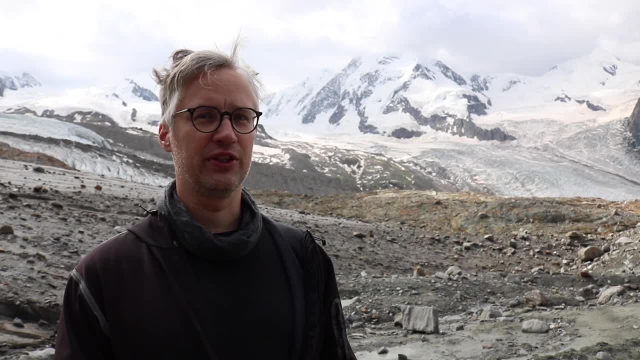 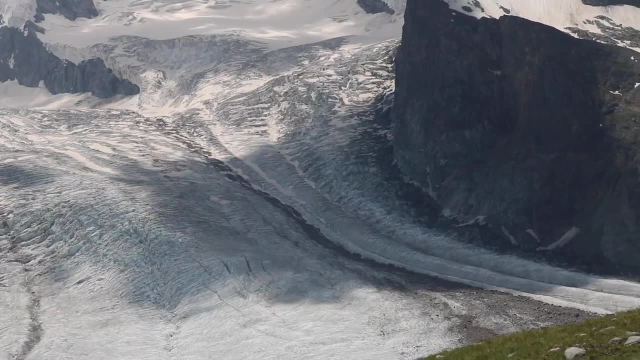 and we have to do something about it. I can't imagine any more fulfilling work. honestly, If you're in a place like this, you see nature. It's almost a spiritual experience for me. You see how humans are really part of nature.